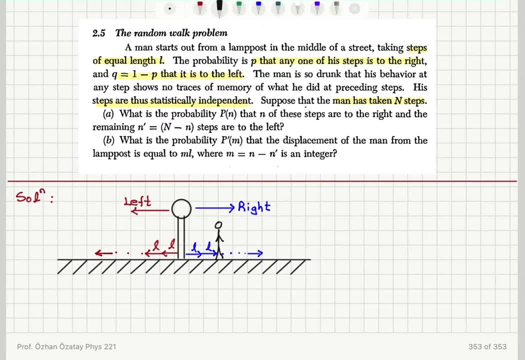 Now we call capital N, that is total number of steps, and he is taking n numbers of steps to the right and N prime number of steps to the left, and we have. So we have n plus n prime is equal to capital N. or we can write: n prime is equal to the total number of steps minus the number of steps he has taken to the right. 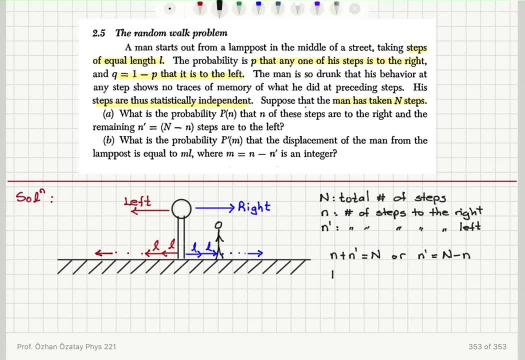 And we call P probability of right, probability of a step to the right, And Q is the probability of having a step to the left. And because we have to have a step, it's either to the right or to the left. P plus Q must be equal to one. 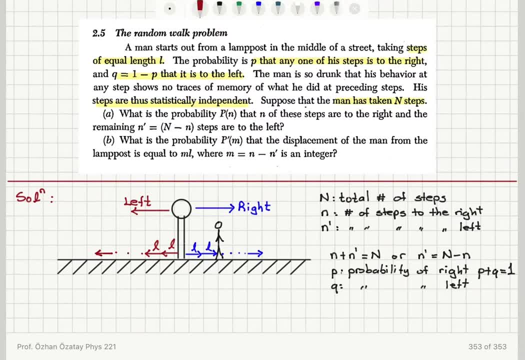 So the probability is normalized. So the answer to question A: what is the probability that n of these steps are to the right and the remaining are to the left? So we're looking for P of n. So what we have to do is we have to choose. 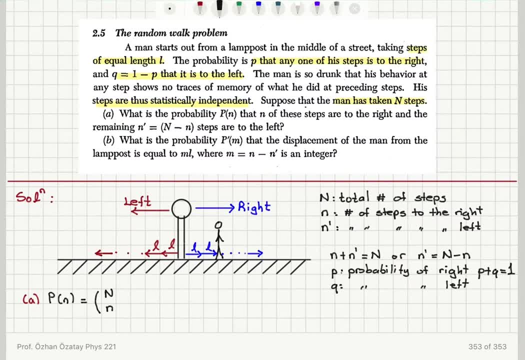 out of capital N's and N prime's, n steps which are to the right. So in how many different ways we can do this and the probability. so, after we have chosen n steps to the right, for each step, the probability is P. 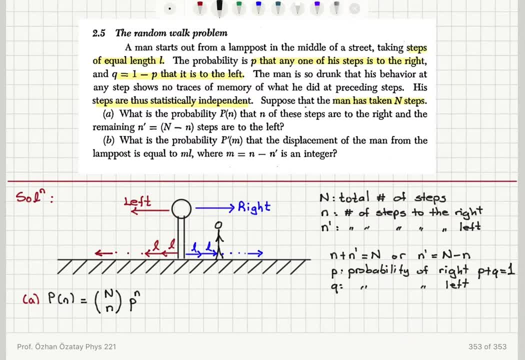 So P to the N will be having n of those steps to the right and the remaining at the same time with probability Q and the remaining at the same time with probability Q and the remaining at the same time with probability Q should be n prime times to the left. so p to the n, q to the n prime. this is our binomial distribution. 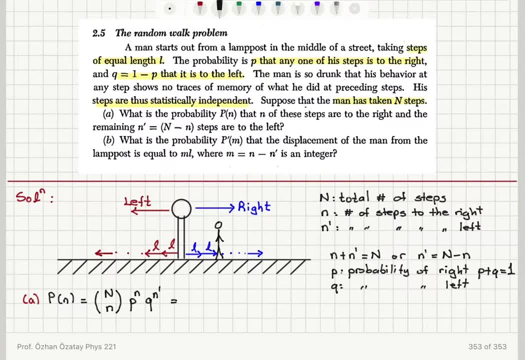 therefore, the answer is going to be given by the binomial distribution, which is: capital n factorial, n factorial. capital n minus n factorial. the number of distinct ways i can choose: n steps out of capital, n steps to the right, multiplied by p to the n and steps to the. 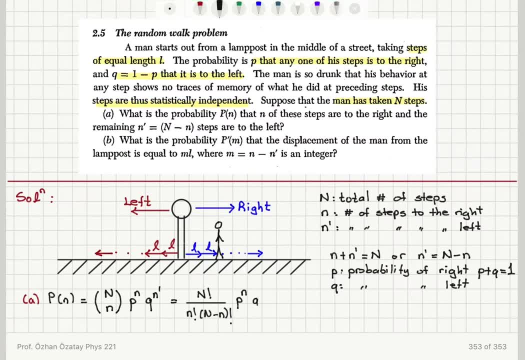 right with probability p and q to the n prime, which is capital n minus n. so this is basically the answer to part a of the problem. now i can answer part you b. what is the probability that the displacement of the man from the lamp post is equal to m times l? 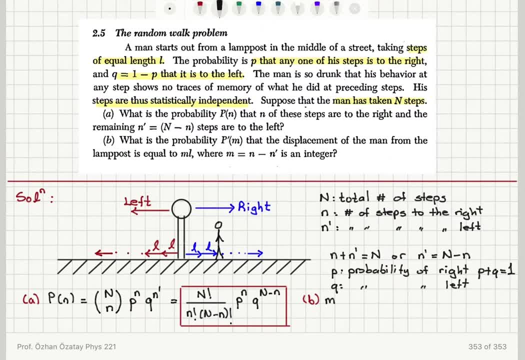 now, m is the difference between the steps to the right and steps to the left and we have we have n minus n prime, which is capital N minus n. so this will be equal to n minus n. so if we are looking for probability of having a value for m, it's the same thing as probability of having a value for n, because M is just 2n minus a constant capital N, which is the total number of. 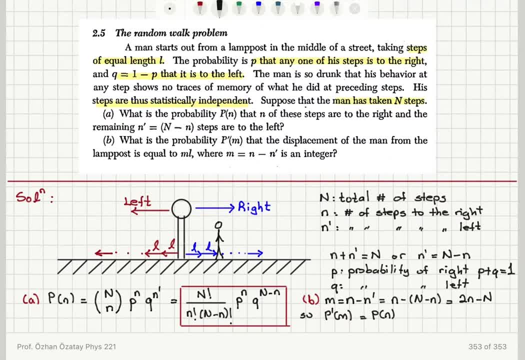 steps. now all I have I have to do is to rewrite probability distribution for n in terms of m. so from this equation that m is equal to 2n minus n, i can write: n is equal to m plus capital, n divided by 2, and since n prime. 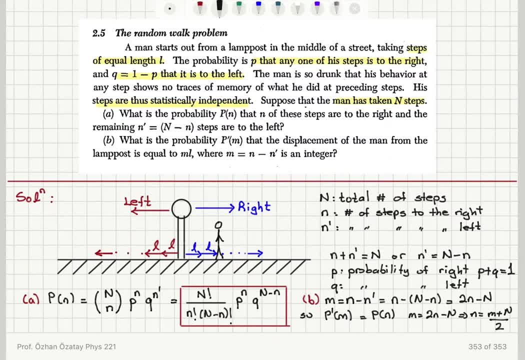 is capital n minus n, and similarly i can write: n prime is equal to capital n minus m plus n over 2, which will give me, for n prime, a 2n minus n capital n minus m divided by 2.. therefore, the answer that i'm looking for, 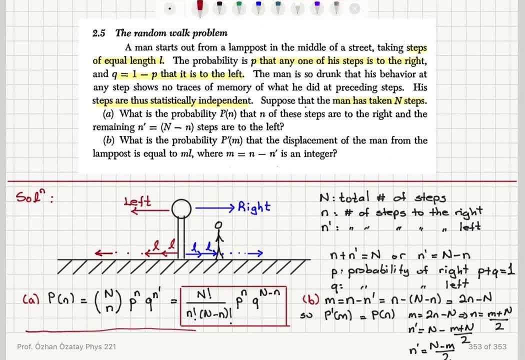 here. so let me separate this. the answer that i'm looking for in part b is p prime of m. is capital n factorial. for n factorial, i'm going to write uh n plus m divided by two factorial. and for capital n minus n, which is n prime factorial, i have capital n minus m divided. 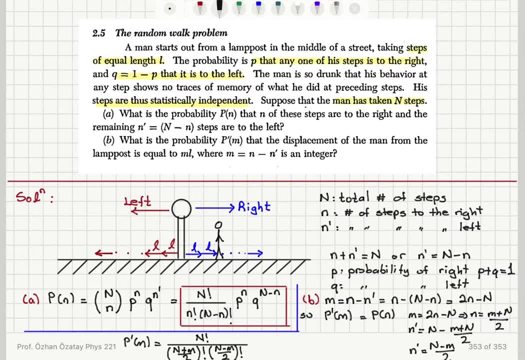 by two factorial, and p to the n. so it's going to be p to the power, n plus m divided by two, q to the power, uh n prime, which is capital n minus m divided by two. so this will be the answer to part b. okay, so we're talking about 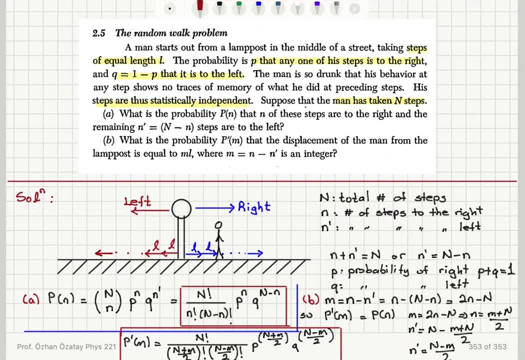 a random walk problem. a man starts out in the middle of a street from a lamp post and is taking steps of l equal length either to the right or to the left, with no memory of the previous steps. the steps are statistically independent because the man is drunk and the man has taken. 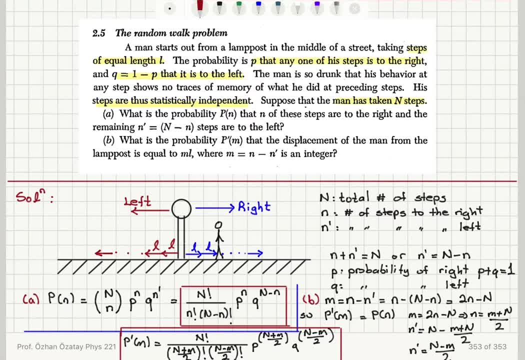 a total of capital n steps. we call the number of steps to the right n and number of steps to the n prime, so that n plus m prime is capital n. total number of steps. p is probability of a step to the right, q is probability of a step to the left, and for each step we have, p plus q is equal to one. 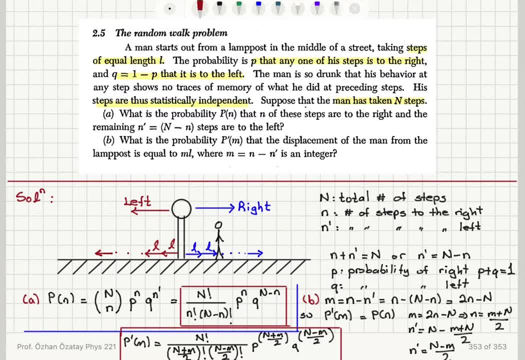 the probability of n of these steps are to the right is out of capital, n steps. we have to choose n steps in a number of distinct number of ways, that is, combinations of capital and objects, taken n at a time, multiplied by probability of a step to the right, to the power n, because